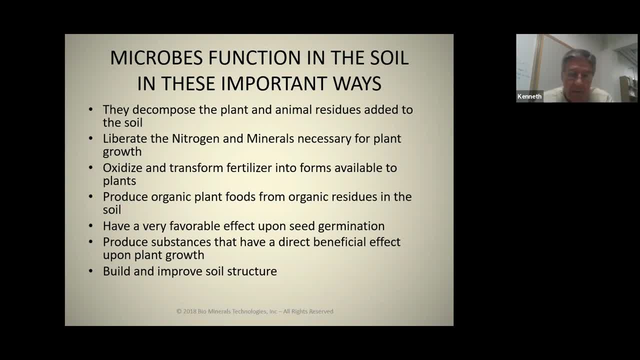 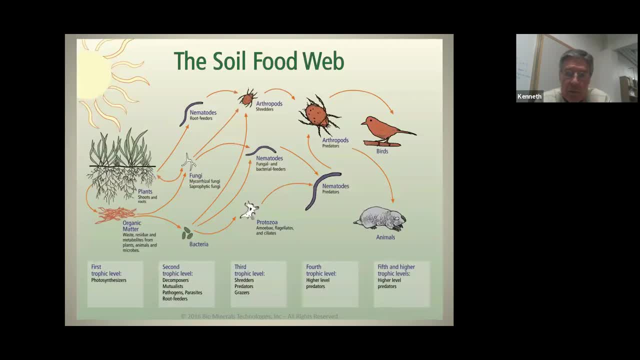 They oxidize and transform fertilizers. They produce organic food. They are incredible for seed germination, Build soil structure, Reduce compaction, Retain water. So we have all of these wonderful microbes in the soil food web. We have all these tropic layers of what everyone is doing. 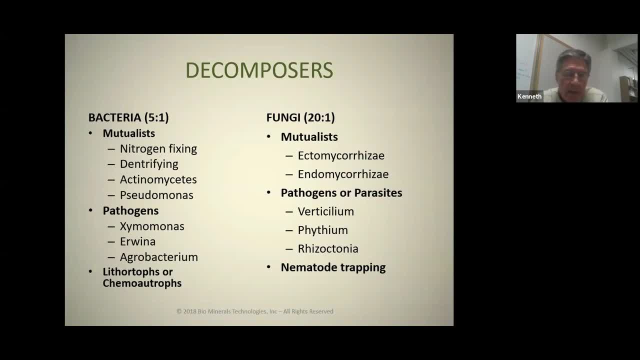 We want to take a look at this, And I want you to pay particular attention to the carbon to nitrogen ratio of these microorganisms, Because this is where God introduces another element of nature, Another element of math, And it's absolutely genius in how this works. 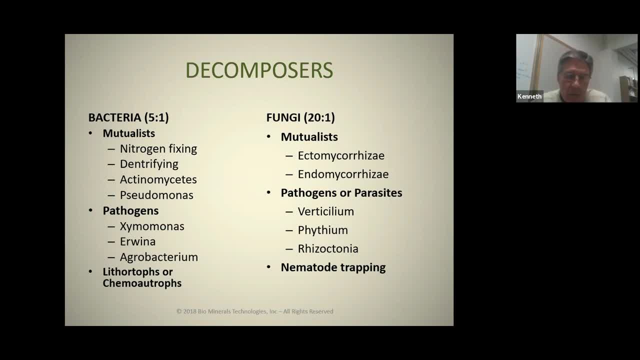 So bacteria in general are five carbons to one nitrogen. And also keep in mind that it isn't just carbon to nitrogen, It's carbon to phosphate, potassium, calcium, sulfur, magnesium, etc. All through the trace minerals. Bacteria are the most nutrient, dense organism on this planet. 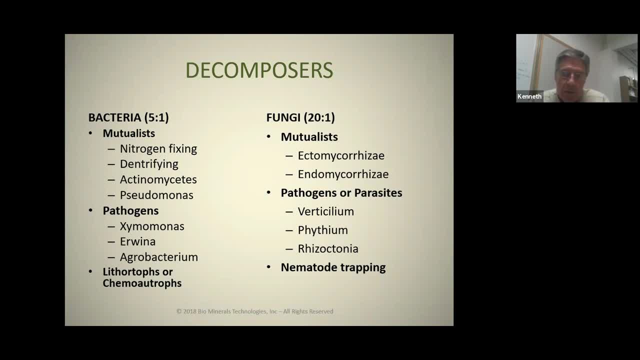 Pure protein is three carbons, one nitrogen. Bacteria as a living organism contain more nutrition than any other form of life on this planet. Fungi are 20 carbons to one nitrogen. We got good guy bacteria, good guy fungi And we got pathogens. 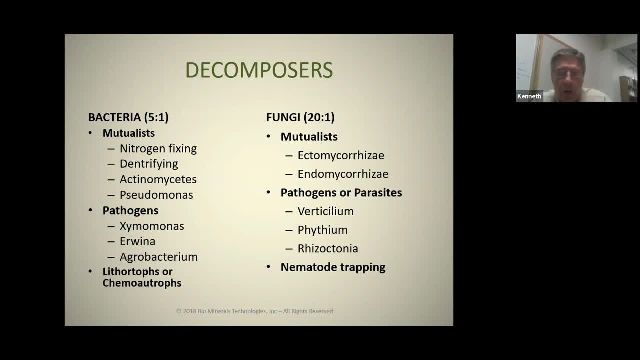 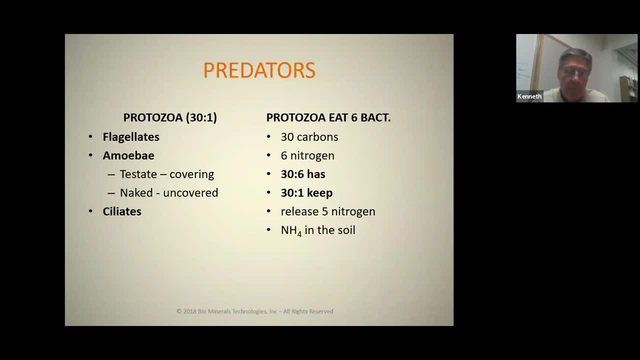 Okay, And the response of the microorganism is who you stimulate, Who you grow, Who you nurture And how you alter the environment to feed them. The next group of microorganisms are protozoa. They are predators. They do not eat and decompose plant material or materials such as animals or other microorganisms. 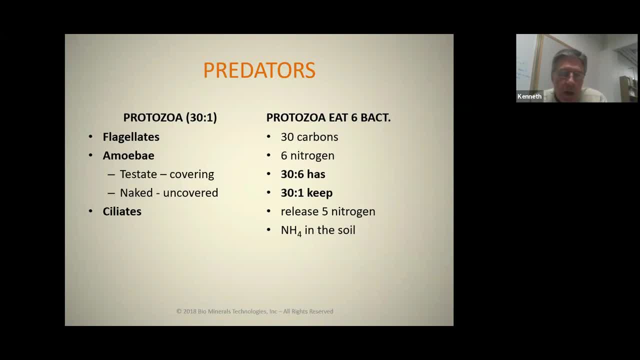 These guys are predators. They're meat eaters. Their job is to eat bacteria. They're 30 carbons, one nitrogen. You and I are 30 carbons to one nitrogen And we eat that which is in our carbon to nitrogen ratio. 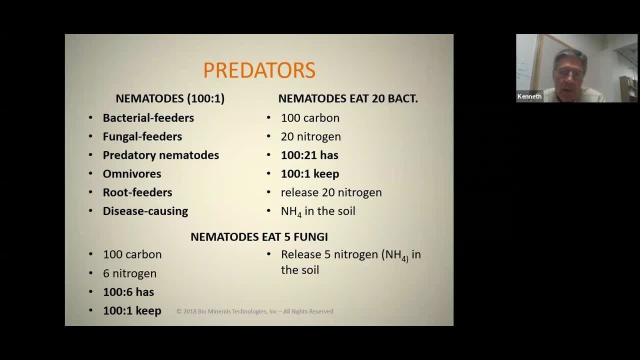 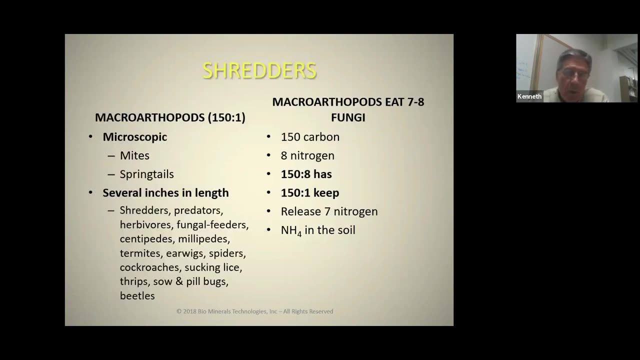 Nematodes, There are 100 carbons to one nitrogen And they primarily eat fungi And that's their job, And we're going to look at how these carbon to nitrogen ratios interplay. Then we go up into our micro and macro orthopods. 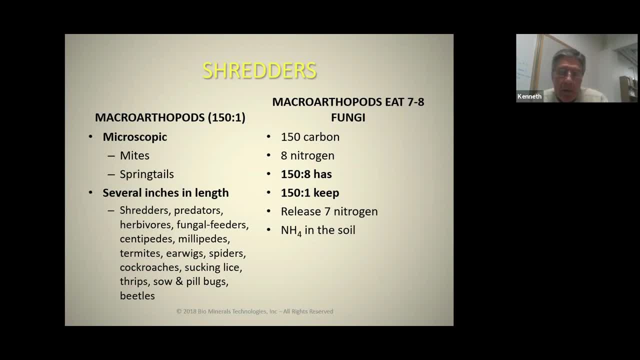 Our carbon to nitrogen ratios get even wider Now. everything in the soil eats something. Everything in the ocean eats something. Every life form on this planet eats something, And so we're all eating off of these food chains. This is how God arranged the cycling of nutrition. 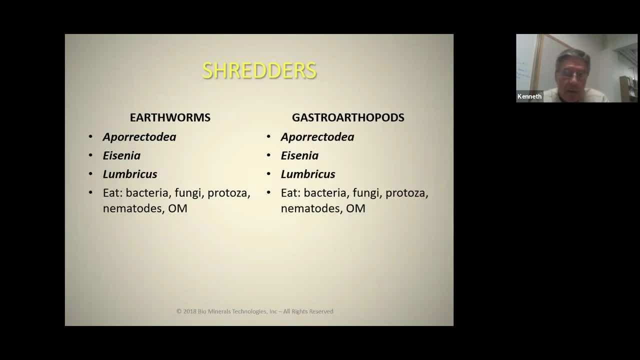 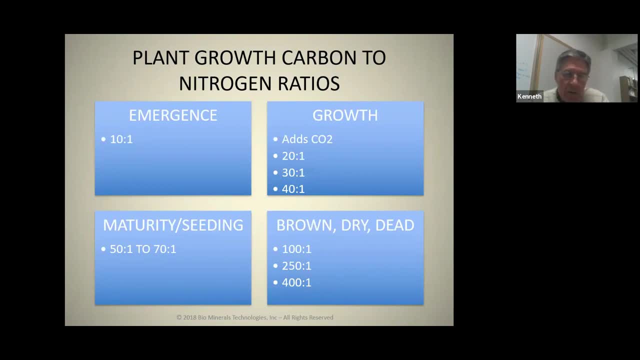 We go up into earthworms, gastro-orthopods, We go up to reptiles, mammals and birds, And so, as plants emerge, there could be 10 carbons to one nitrogen. As they grow, they're adding way more carbon dioxide than they are nitrogen. 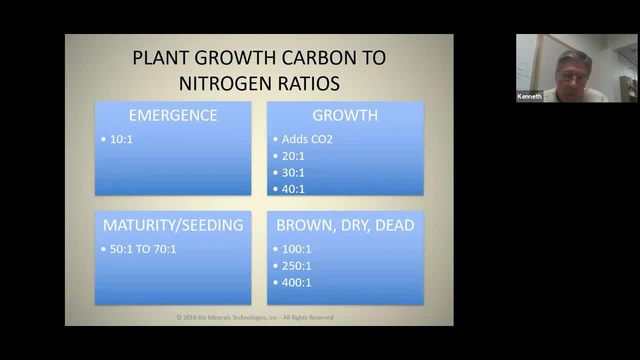 And so when a plant gets up there, when a plant gets into maturity and seeding, it can be 50, 70, 80 carbons to one nitrogen. When they're dead and senescent they're upwards of 100 to 200 to 400 carbons to one nitrogen. 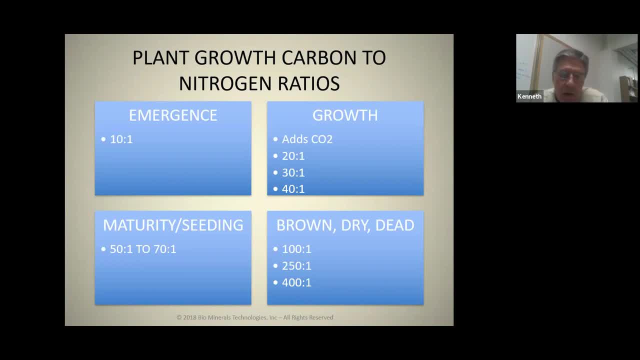 When you watch a cow graze in the field. they don't want the tall grass, They want the short grass, Because the carbon to nitrogen ratio is at their ratio or less. They're smart enough to understand that if they're at 30 carbons to one nitrogen 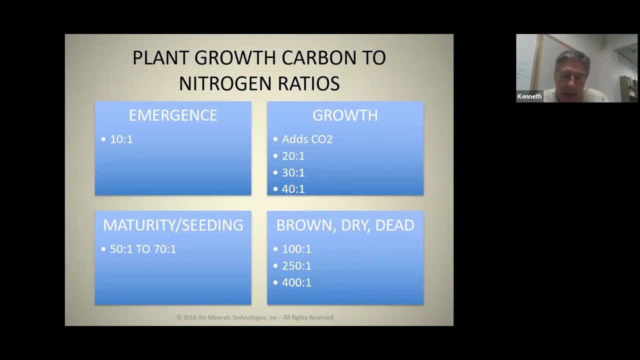 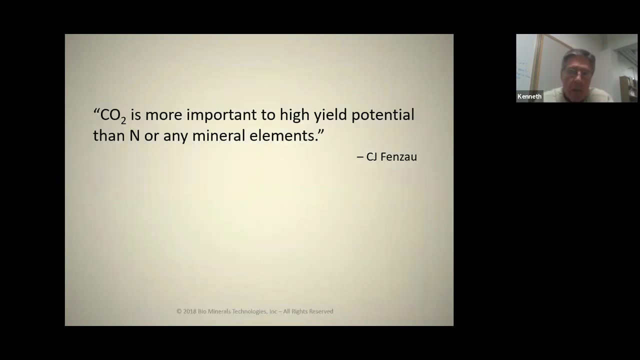 they're not going to live and maintain their ratio eating 50 or 70 carbon to nitrogen ratio material, So they don't touch it. We're the same way. We like those things at or near our carbon to nitrogen ratio. CO2 is more important to high yield potential than N or any other element. 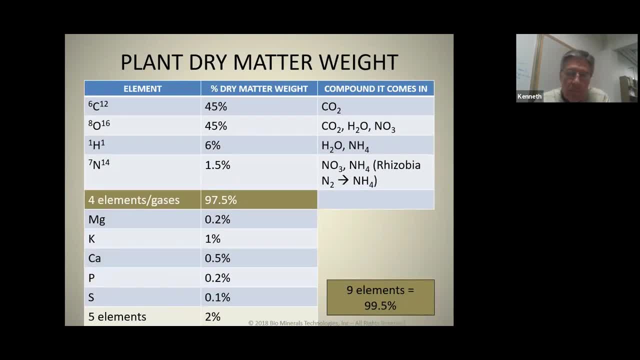 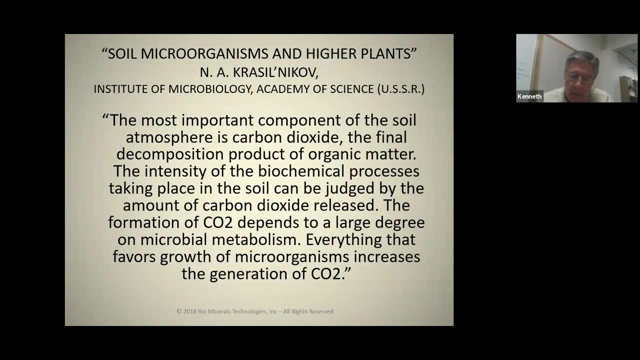 And again we're going back to carbon oxygen, and it's 90% present in plant dry matter. We talked about this earlier. Carbon dioxide is what is produced by microorganisms and that is the basis of your plant biomass. It is actively taken up by the roots. 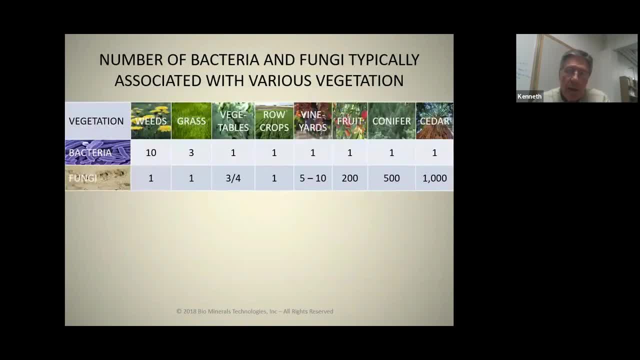 The more of it you have, the faster your plants will grow. Every plant that we grow out here has a proper bacteria to fungal ratio. If we want to encourage weeds, we just put in high bacteria. The vegetables, the row crops are about one to one ratio. 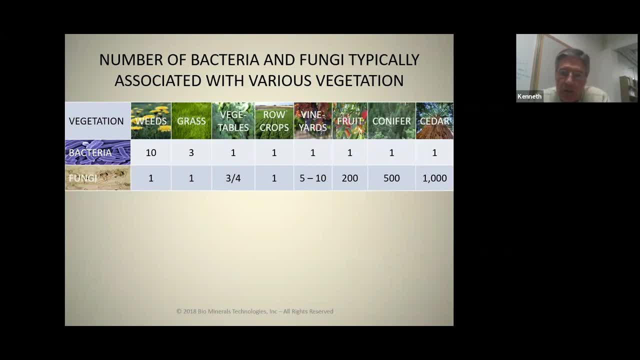 one bacteria to one fungi. In addition, as we get into woody plants they now become fungally dominated, to where our vines are five to ten fungi to one bacteria. Our fruit trees can be as high as 200 fungi to one bacteria. 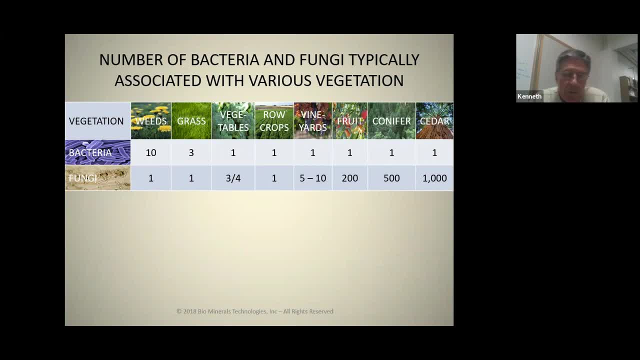 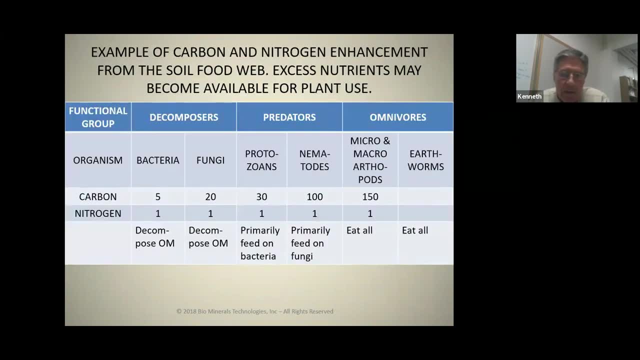 Conifers 500 and old growth for us up to 1,000 fungi to one bacteria. So when we're growing plants we've got to make sure we get the right microorganisms underneath these plants so that they feed the plant property, because some plants are alkaline in nature. 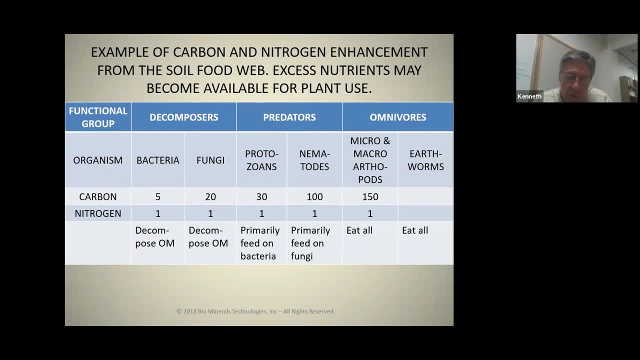 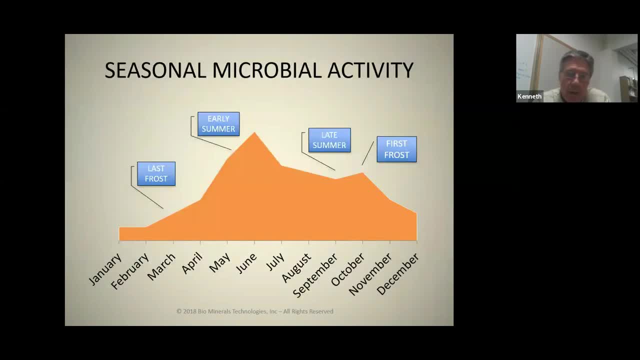 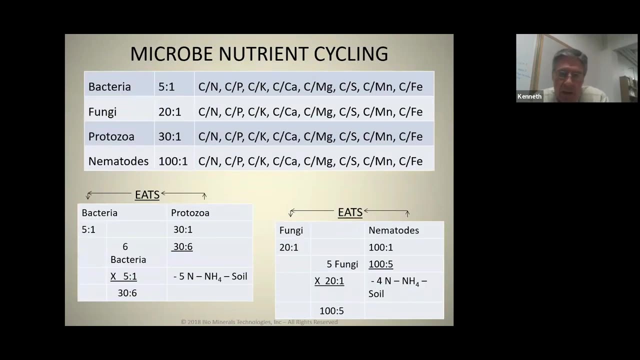 and they need an alkaline soil which comes from bacteria. Other plants are acidic in nature and that environment comes from the acidic strands of the fungi. Our microorganisms are going to parallel our plants' growth season perfectly. So here's where God's math comes in. 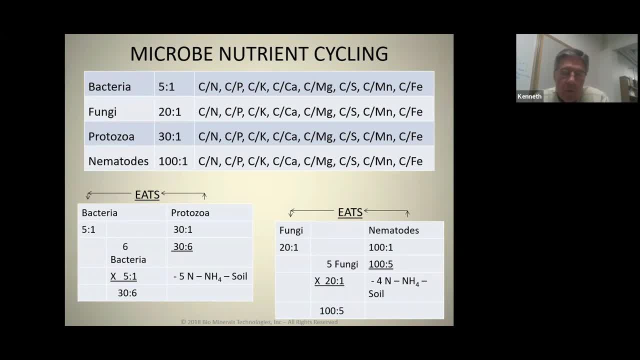 and how nutrient cycling occurs in the soil Bacteria: five carbons to one nitrogen, But it's also potassium, phosphate, calcium, sulfur, magnesium, iron, manganese, copper, zinc, boron, cobalt, all the way down the line. 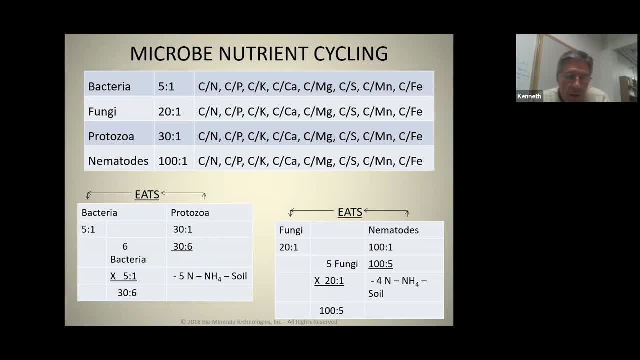 Fungi, 20 to one, 30 to one, So protozoa come over and eat bacteria up to 10,000 a day. For a protozoa to maintain 30 carbons and one nitrogen, he has to eat six bacteria at five to one. 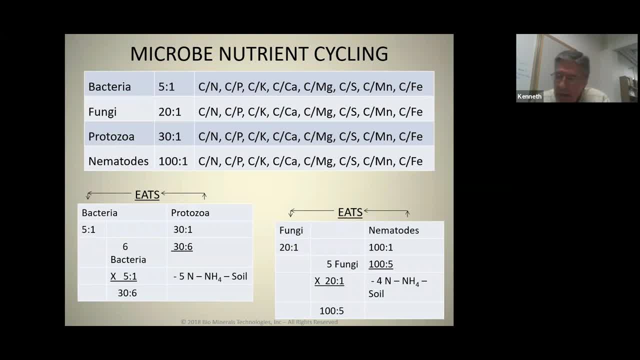 But at that point he also has six nitrogen. He can't keep six nitrogen, He has to excrete five nitrogen back in the soil, Goes back out as NH4, ammonium and the plant takes it up because the plant is putting out sugars. 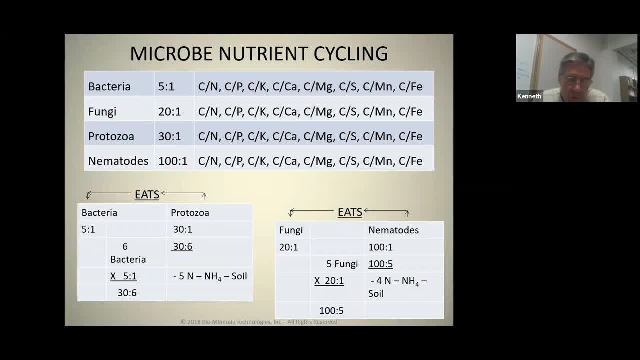 the microorganisms, the bacteria and the fungi go to the root, start multiplying and the protozoa come in and start eating the bacteria. The nematode eat the fungi. The mineral release is on the root system for the plant. 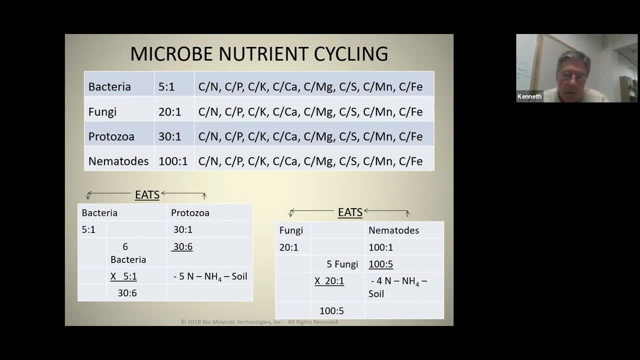 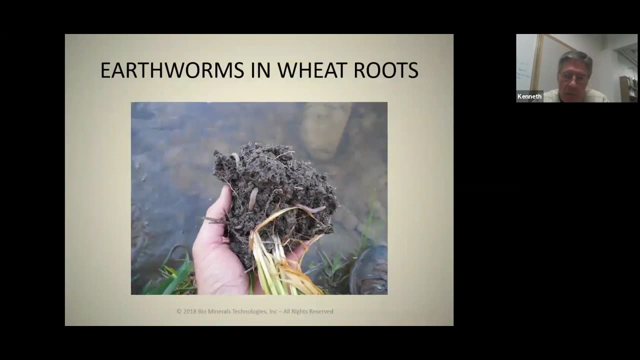 So again, it is a larger organism eating a smaller organism, a lower carbon-nitrogen ratio, excreting the difference. And this is how God maintains the prairies and the plains and the forests. In all of our soils we have all these tropic levels of microorganisms. 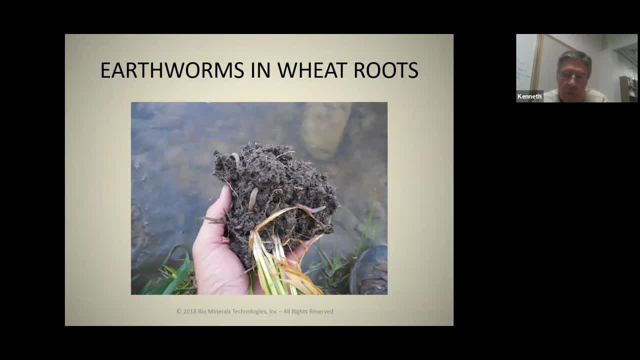 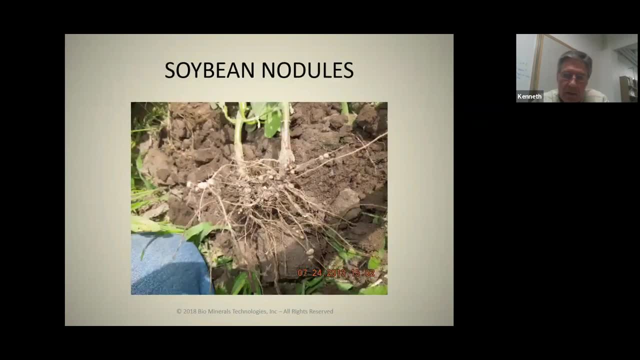 Earthworms won't be there unless everything underneath them in the food chain is present, And we want these microorganisms because they're eating and they're releasing nutrients for our plants. These are soybean nodules, So just a single ripe plant. 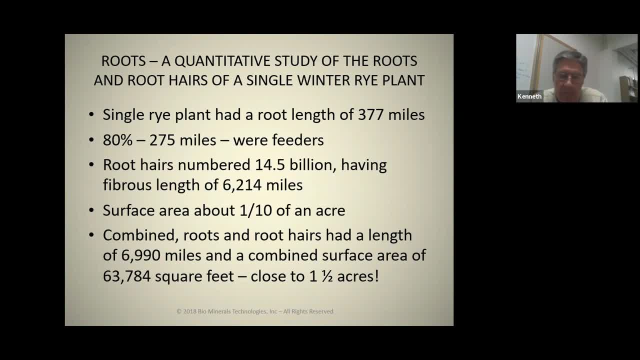 We start looking at how God creates infinity in a finite area. This was also done by the Russian study. A single ripe plant root length has 377 miles. 80% of that were feeder roots. The reason it took two years to complete? because they had 14.5 billion roots. 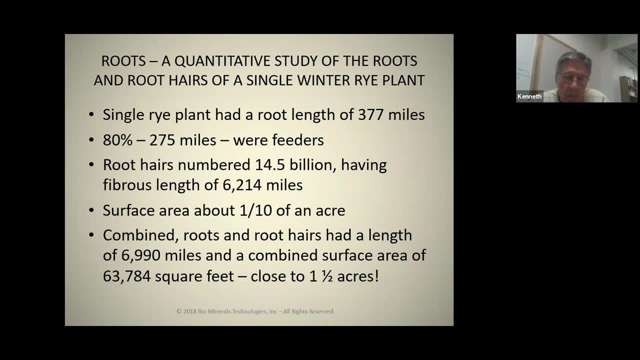 Their fibrous length is 6,200 miles. When you combine the roots and the root hairs, we had almost 7,000 miles, or an acre and a half of surface area. Again, these plants have incredible intelligence. They have incredible presence. 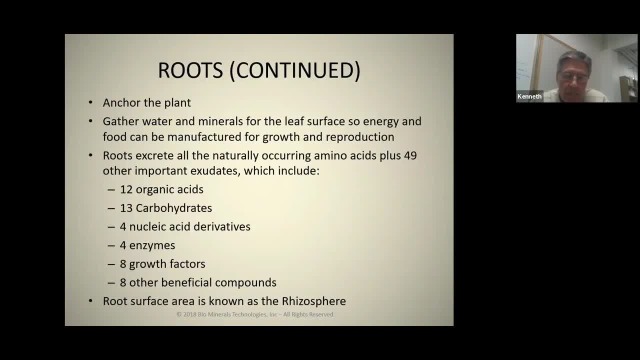 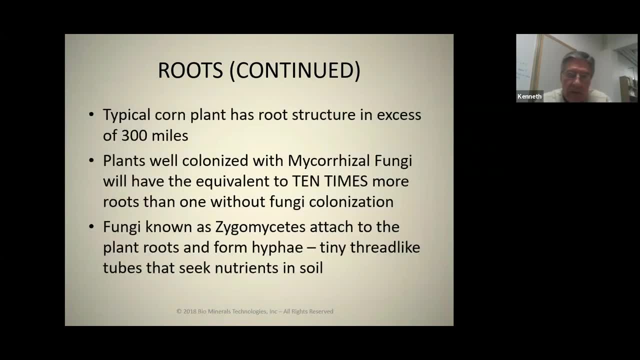 Plant roots produce exudates from photosynthetic compounds. They feed the microorganisms And that is the intelligent communication between plants and soil biology. Corn plants have approximately 300 miles of root And mycorrhizal fungi who can enter seed into the root. 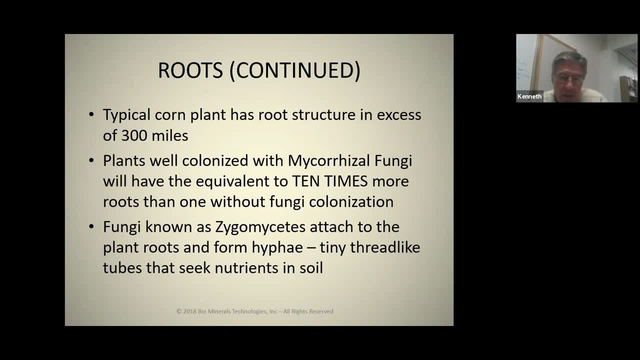 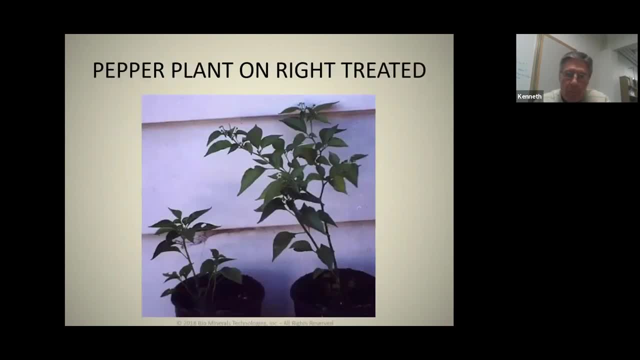 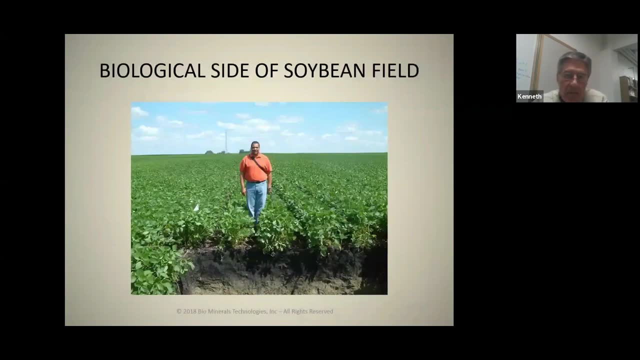 and infect it and grow from the nutrients provided by the plant can increase the root equivalent In the soil by tenfold. Plants with biology, plants without biology: This is a field in Minnesota where we have soybeans being on the biological side. This is a transitional side. 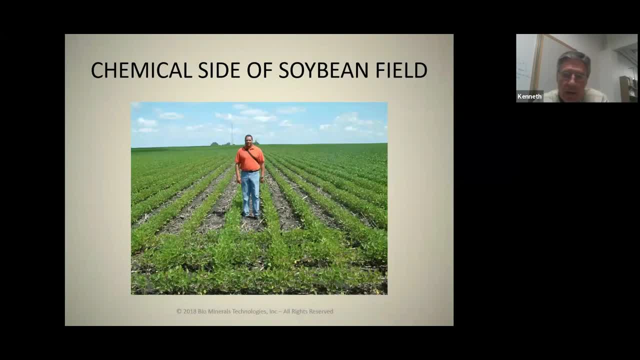 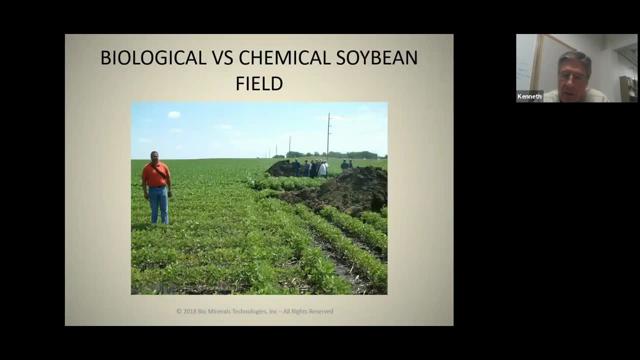 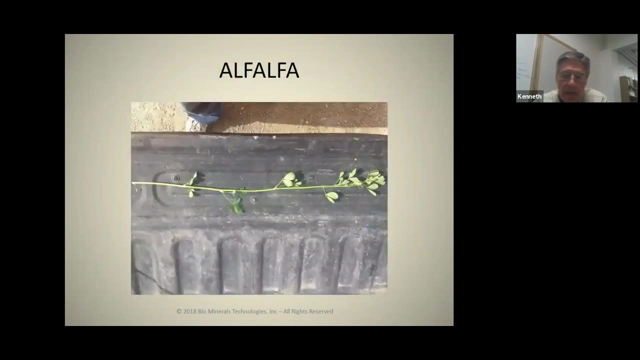 This is the chemical side. You simply look at the plant and you get the biological response. There's only 150 feet between the chemical side and the biological side. Here's a corn plant with six ears. This is an alfalfa plant with approximately nine nodes. 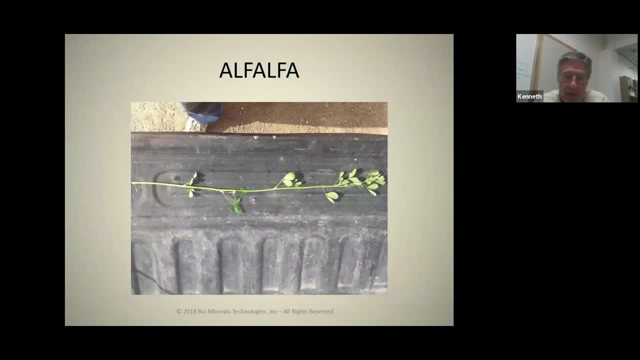 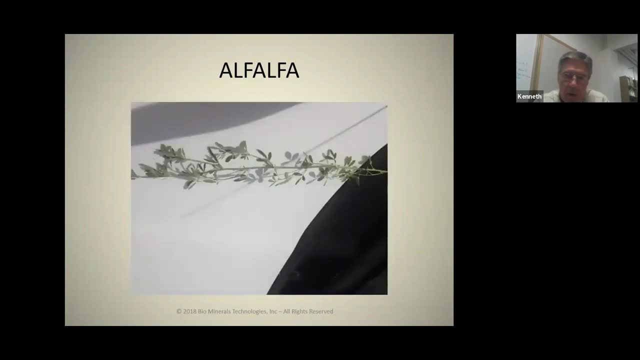 And in this stem there are dozens and dozens and dozens of potential nodes, but they're not activated With some mineral and microbial nutrition. 100 feet away, in a different part of the field, the same plant will produce 17 functional nodes and more leaves. 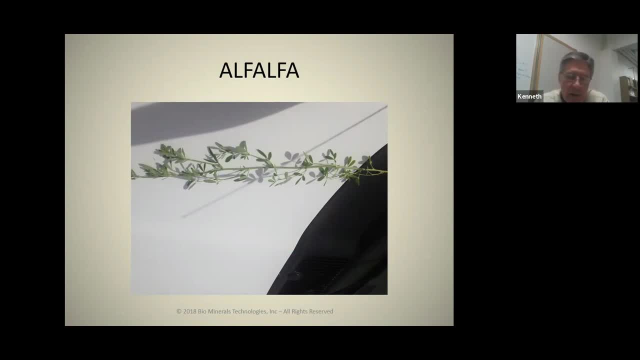 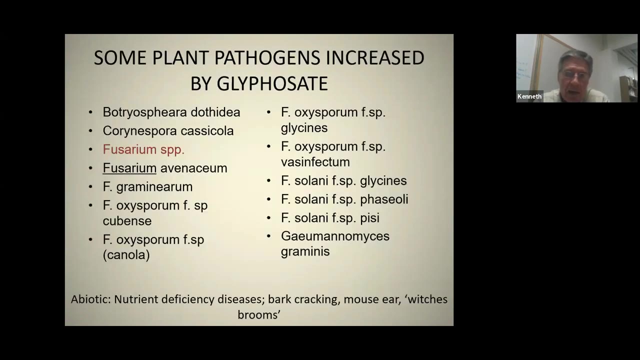 So the potential in the plant is dormant unless there are nutritions and trace elements supporting the nodes. We currently have up to 27 nodes pushing out branches and leaves on alfalfa plants, And there's more in there. We haven't learned how to get them out yet. 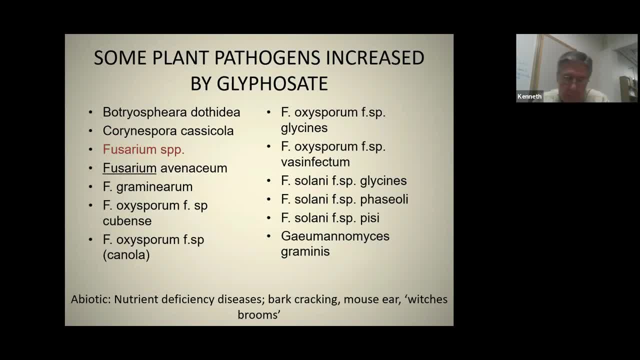 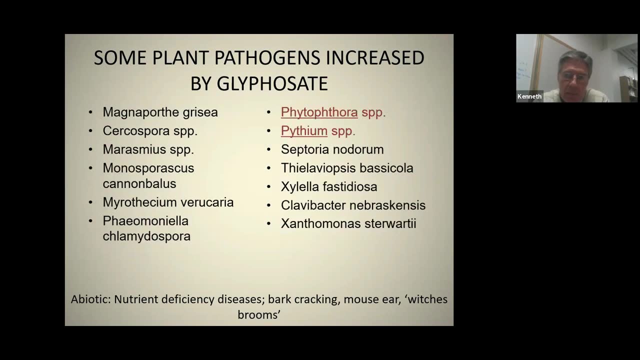 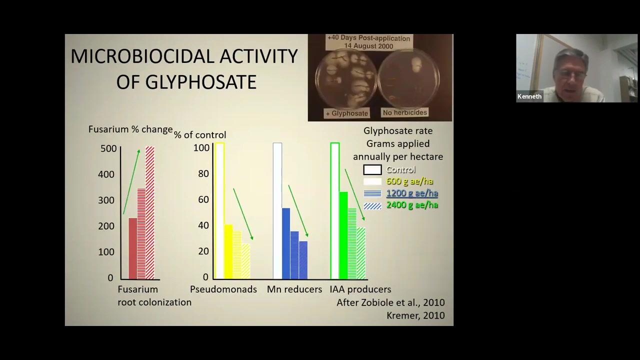 Glyphosate is a massive suppressor of good organisms and it stimulates the pathogenic organisms, Whether it's Phytophthora, Pythium, Fusarium. So when you apply glyphosate at various rates, what you're going to see is a massive increase in your pathogenic populations. 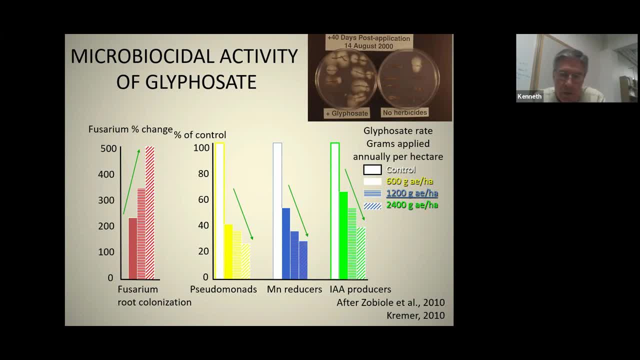 and you're going to see a strong decline in your Pseudomonas, your manganese reducers and your beneficial microbes across the board. Roundup will, at one-tenth of one part per million, will begin affecting beneficial microorganisms. It takes up to 4,000 times more glyphosate to kill pathogens. 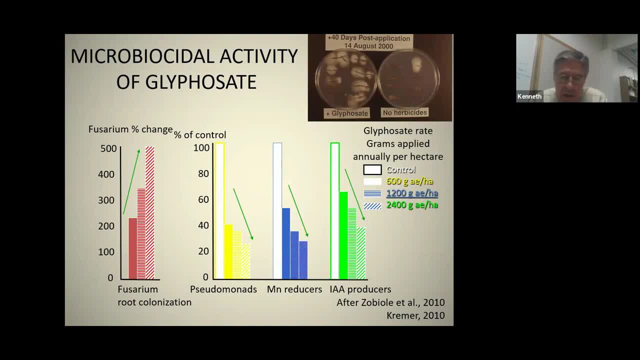 And so your glyphosate compound is a very, very potent antibiotic, specifically on the beneficial microbes first, And that's why we see such a massive switch in soil populations. when we apply glyphosate, We're decimating our beneficial soil microorganisms. We're destroying that life and health in the soil. 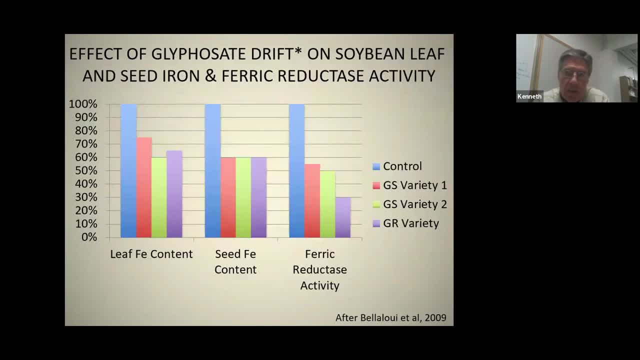 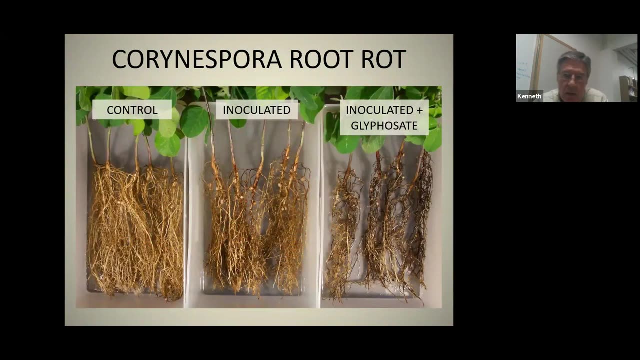 and we're absolutely exploding our pathogenic populations. We also lose our mineral components in our plants. We can see the difference in the plant roots. as far as disease response, Glyphosate by itself cannot kill a plant. It can stunt a plant. It will pull the positive trace minerals away from the enzymes. 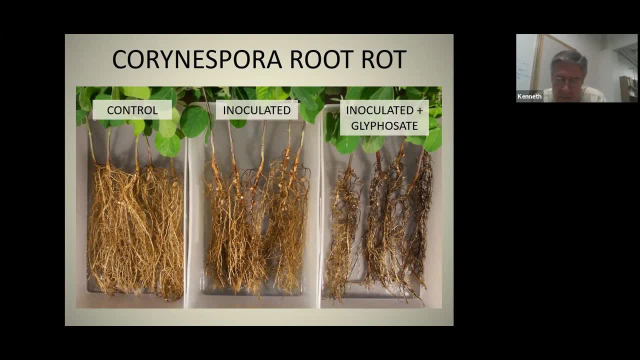 and shut the plant down. Glyphosate is phosphate-based, It is negatively charged and it's going to electromagnetically pull the trace elements and it shuts the plant's defense mechanisms down, Having killed the beneficial microorganisms in the root systems. 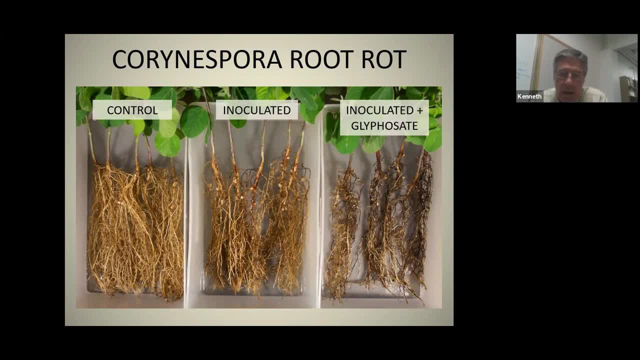 the pathogens then come back in and they attack the root, And so you have a two-step mechanism with glyphosate or Roundup working. One, you shut the plant down. The second one is you kill it with a pathogen, And that is the process by which glyphosate works. 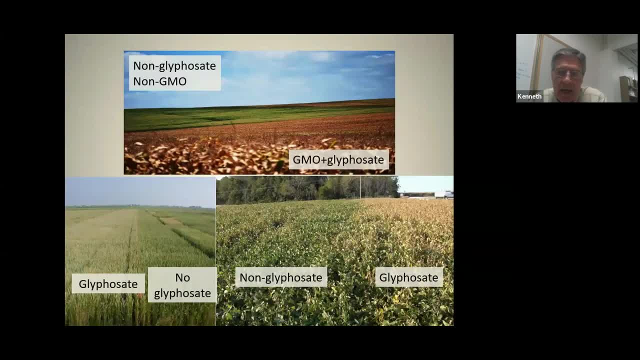 You can see, in these fields where you have glyphosate-induced mineral deficiency, These soybeans have turned bronze because the manganese and the magnesium have been chelated by the glyphosate and the plants will not get their green back until they replace that mineral they lost in the glyphosate applications. 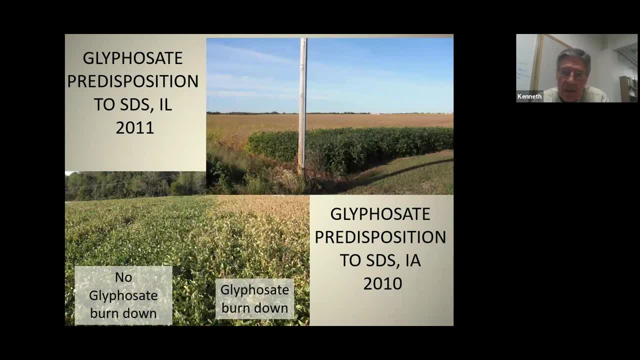 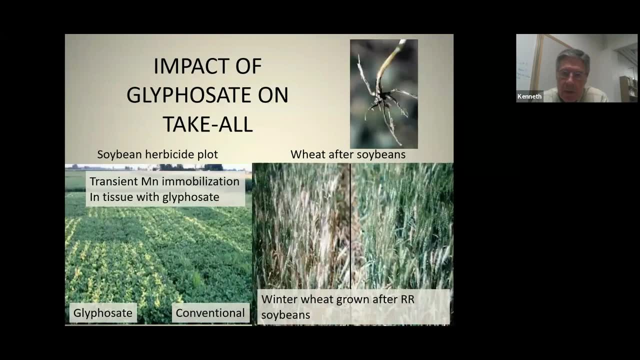 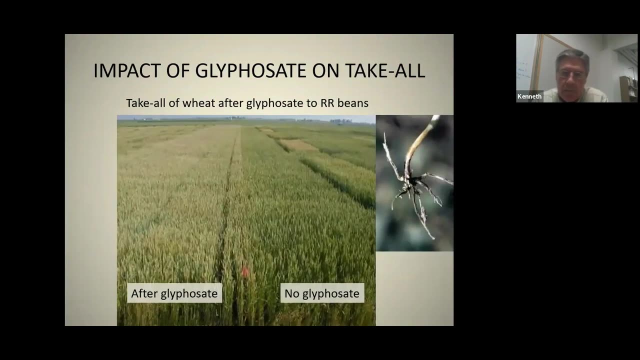 Right here you can see where they didn't spray these particular soybean plants and they're still green and functional. Everything else had the minerals taken away from it. You have a whole series of diseases. You can see the mineral loss which will weaken the plant. 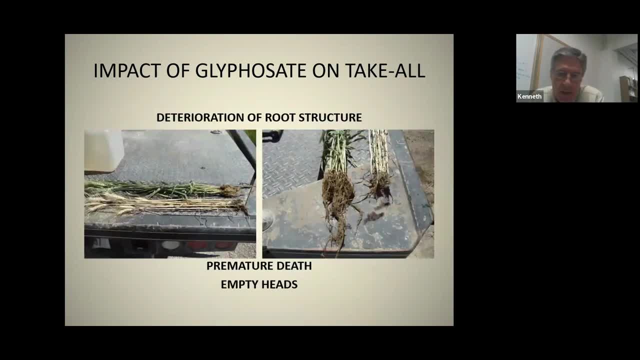 These are some farms that I had worked with up in Montana. They were spraying a lot of glyphosate. It brought on a disease called take-all disease, where the pathogens would go in and destroy the root systems and the plants would die early in maturity. 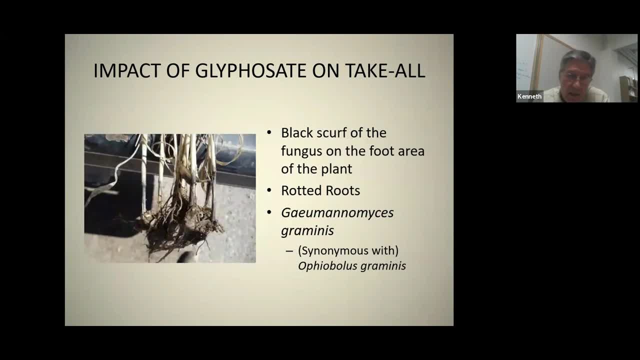 and there'd be no grain in the heads. So you can see the blackening of the crown and the loss of the root system. This particular pathogen is responsible for this and it's just overstimulated by the presence of glyphosate. 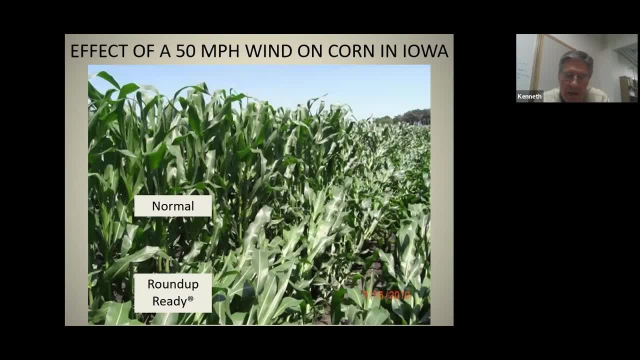 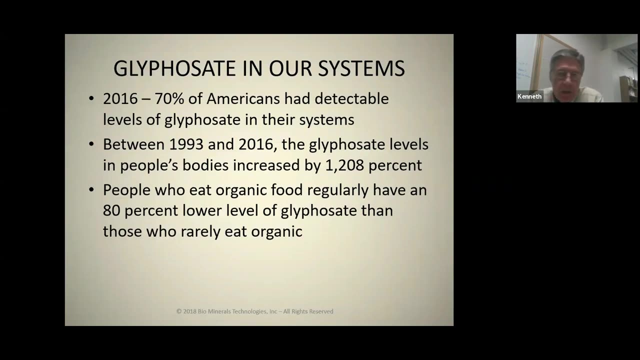 In Roundup Ready corn because it chelates the copper and the manganese. the polyphenol oxidase enzymes do not put these stocks together as strong as they could be and they go down in wind. Glyphosate in our systems: in 2016,, 70% of Americans had detectable levels of glyphosate in their system. 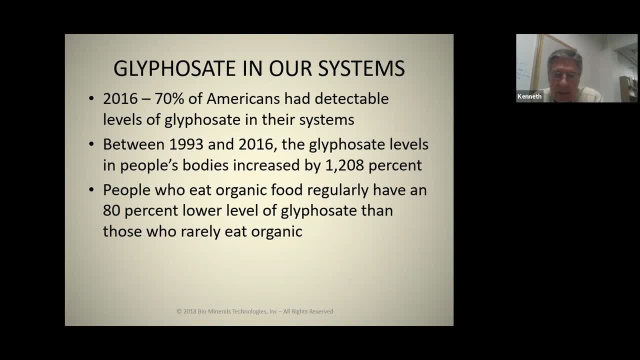 Between 1993 and 2016,. glyphosate levels in people's bodies increased by 1,208%. They found that people who regularly ate organic food had 80% less glyphosate than those who rarely ate it. Glyphosate is prohibited in the application in organic food production. 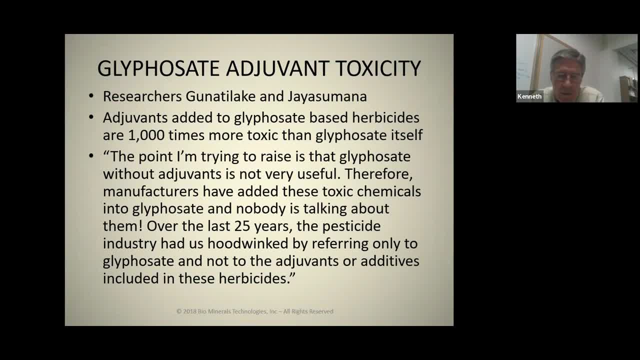 These two researchers from Sri Lanka, who were determining the kidney disease that was happening to the cotton workers, where they were losing approximately 25% of the field workers, noted that the adjuvants added to glyphosate-based herbicides are 1,000 times more toxic than the glyphosate itself. 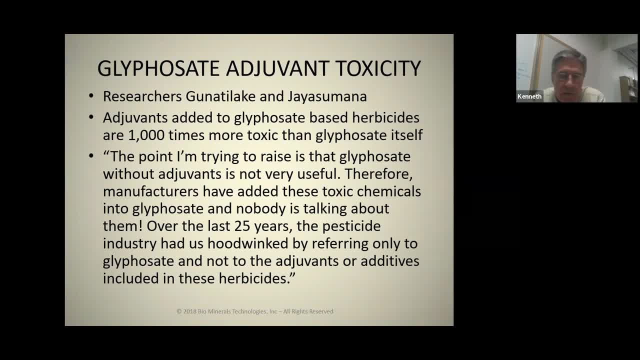 The point I'm trying to raise is that glyphosate without adjuvants is not very useful. Therefore, manufacturers have added these toxic chemicals into glyphosate and nobody is talking about them. Over the last 25 years, the pesticide industry had hoodwinked us. 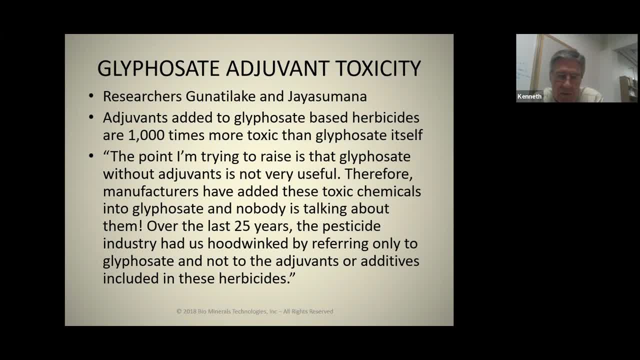 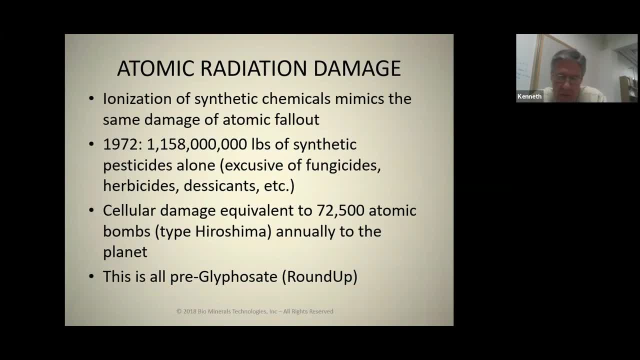 by referring only to glyphosate and not to the adjuvants that were in these herbicides. If you look at the radiation damage, there is a method of calculating radiation damage not only from hydrogen bombs but also from chemical radiation. There was some computation that was done. 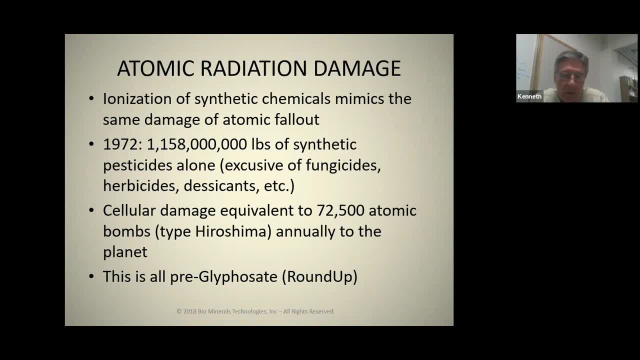 in Italy and it was in the agricultural research scientific area where they were looking at the radiation from chemical damage. They related it back to hydrogen-type bomb damage that we used in Japan to end World War II. You look at this: Ionization of synthetic chemicals. 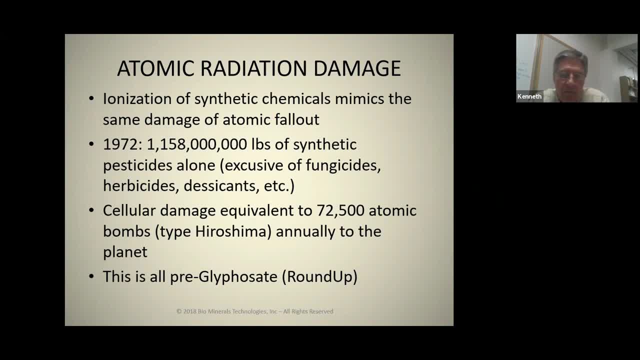 mimicked the same damage as atomic fallout. In 1992, worldwide we were using 1,158,000,000 pounds of synthetic pesticides. Now this is exclusive of fungicides, herbicides and desiccants. at the time, 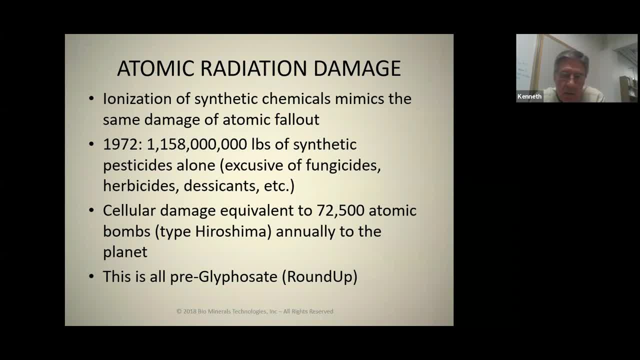 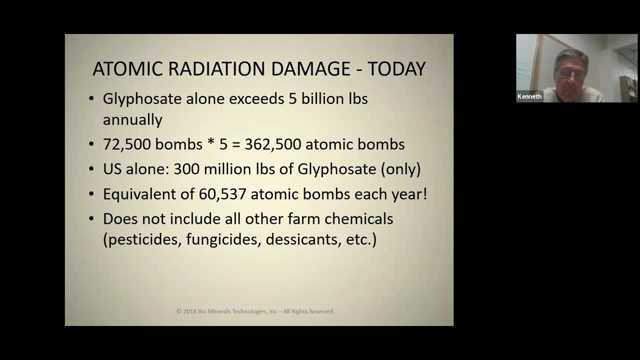 Cellular damage equivalent to 72,500 type Hiroshima bombs annually to the planet. Now, this is all pre-glyphosate. Glyphosate alone now exceeds 5 billion pounds annually. That's five times more than we were using in 1972. 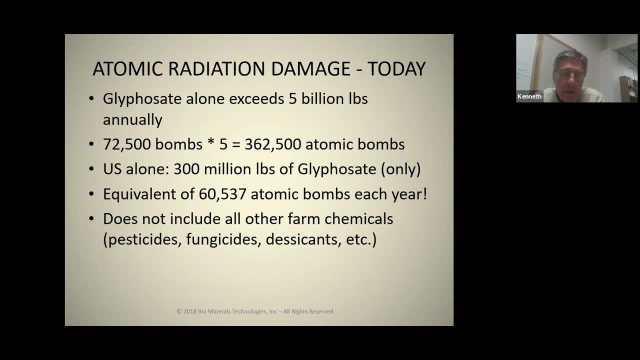 of just pesticides, That is the equivalent now worldwide of 362,500 atomic bombs. You look at the radiation fallout That is exclusive of pesticides, fungicides and desiccants. This is glyphosate alone In the US alone. 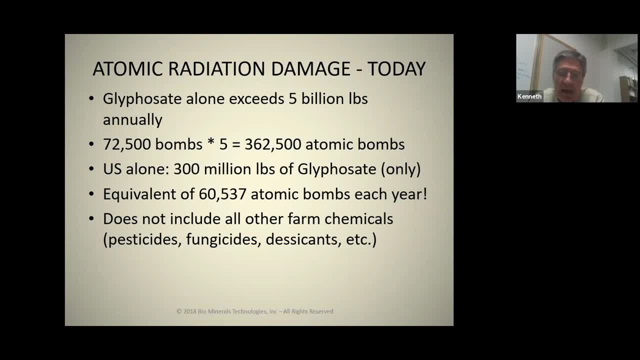 we apply 3 million pounds of glyphosate a year. That equivalent is over 60,000 atomic bombs each year. This does not include the pesticides, fungicides and desiccants that are used in addition to this, And you don't need to ask yourself. 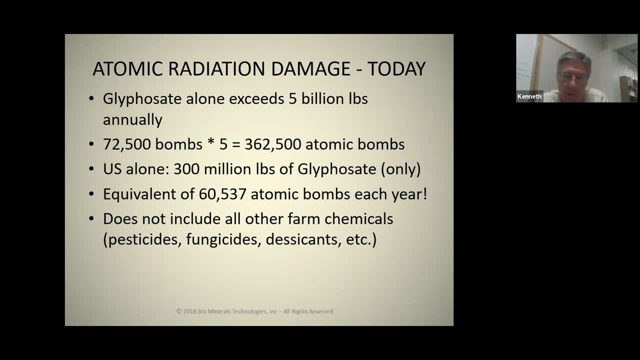 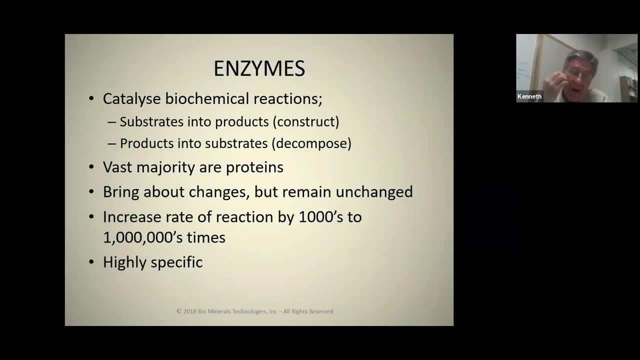 why are we sick? Why is every degenerative disease escalating in this country? Enzymes, these are the marvelous little things in microorganisms, plants, animals and humans. We all come with our own individual enzyme package, And what these do is they put things together. 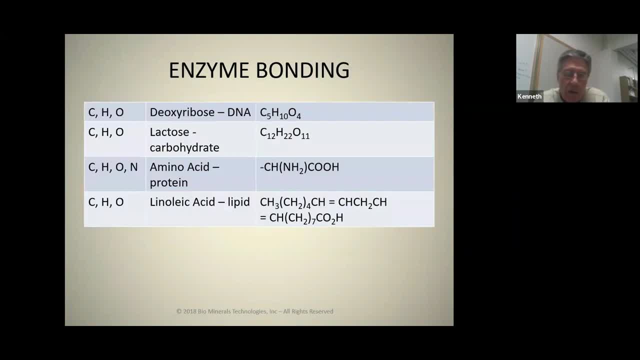 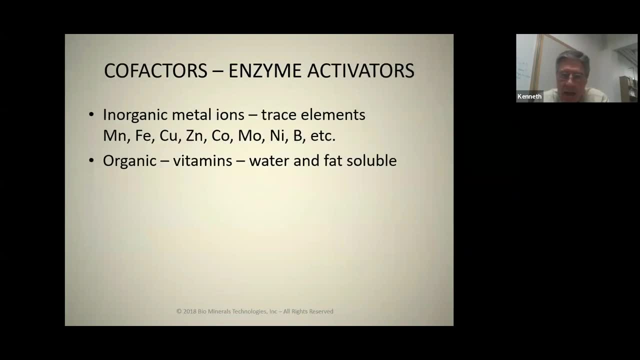 they take things apart and they change these wonderful compounds. Our DNA is made of that. Our carbohydrates are amino acids and proteins, And again we have to have trace minerals, cofactors. to make all this work. Nitrogen has to have molybdenum to go from an element. 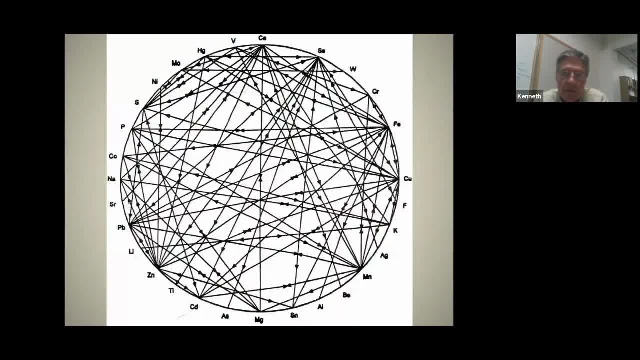 to a compound, to amino acids, to proteins. They're all interactive. Every mineral has to have several dozen assisting minerals to get it there In our soil. microorganisms: we have protozoa, we have nematode, We have good guys. 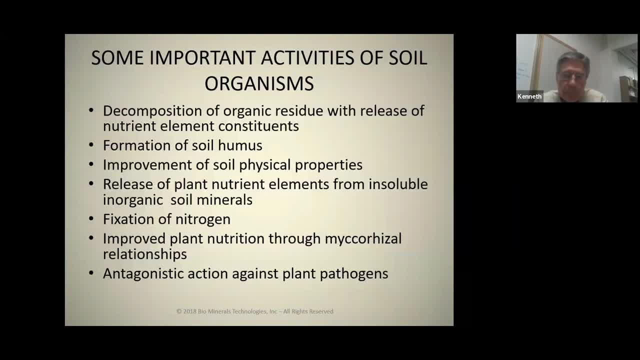 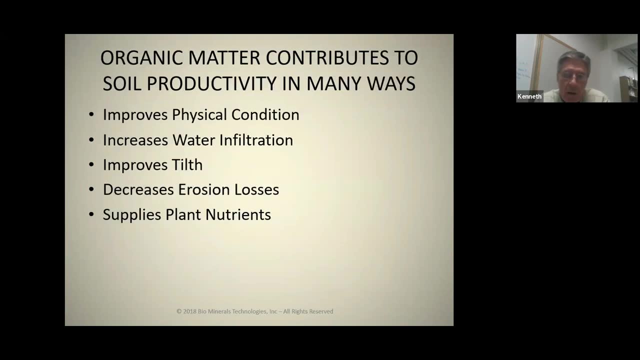 This is an amoeba-eating bacteria. We're going to try to move through this fairly quickly. They decompose organic residue, They form soil humus, They take compaction out of the soil, They fix nitrogen. They improve water filtration, tillage softness of our soil. 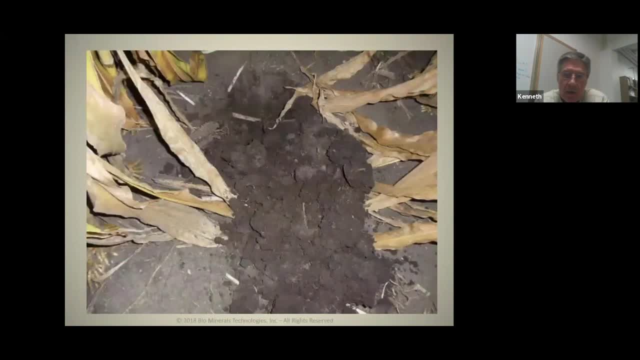 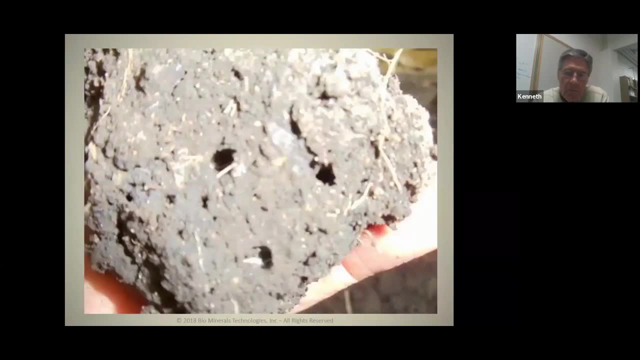 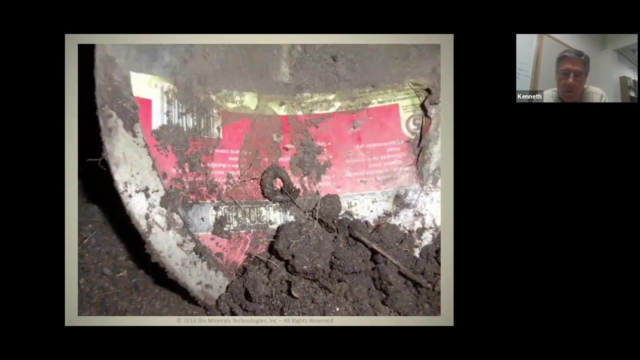 We decrease erosion Crop residue. we put soil microorganisms on corn in the Midwest. We looked at the soil a year later And it's clean. We've got earthworms. We've got earthworm here. We've got holes where the earthworms are moving through the soil. 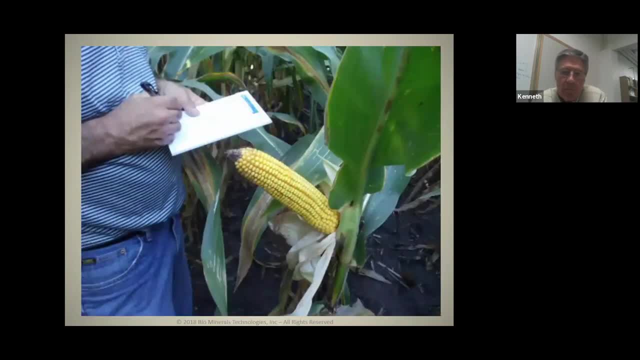 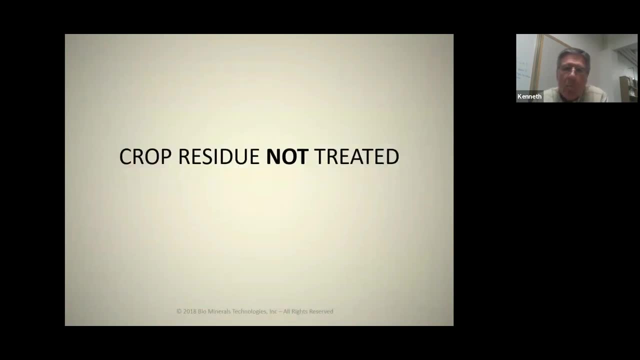 We've got a macro-orthopod And we've got about five rows of tip-back that didn't quite fill on this corn. Let's go into the side of the field 100 feet away. that got no microorganism activity As we started to dig between the rows. 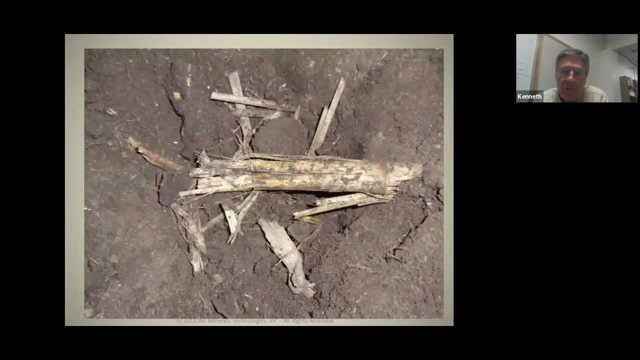 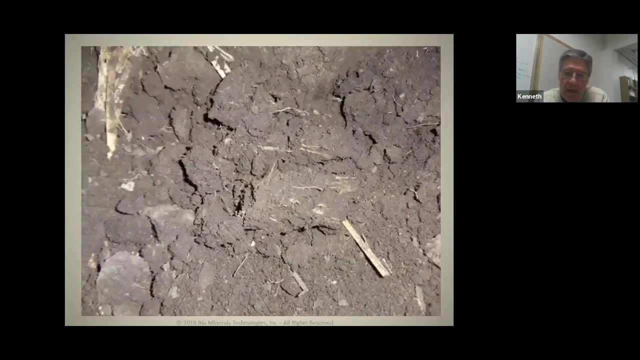 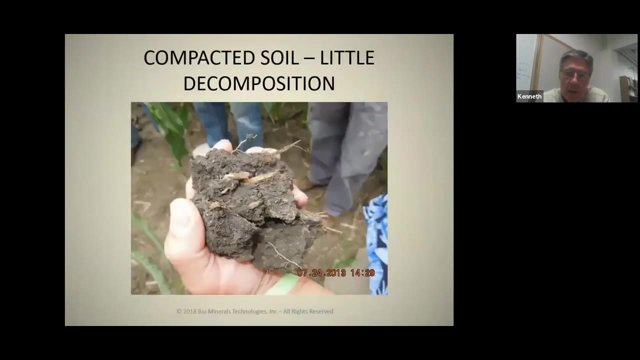 you could see a lot of organic matter still there from the previous year, 11 months earlier. There's been no decomposition of much of the corn material. You can see how the material of the plant is stratified in these clods. You look at this compaction. 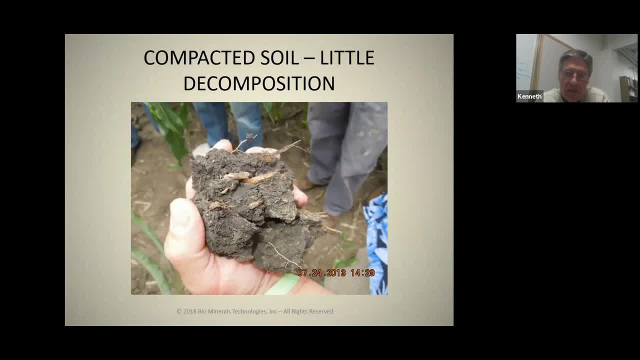 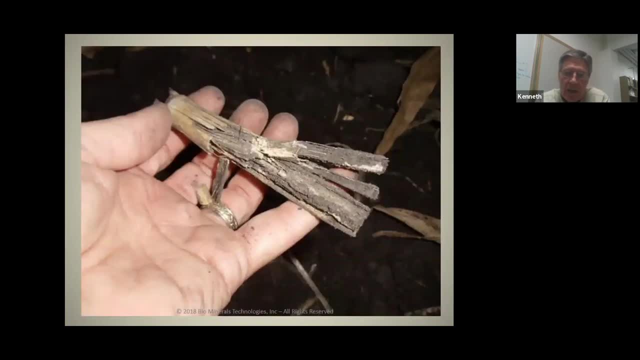 and almost petrified material sitting in these dirt clods. It's not breaking down. This soft pulpy core in the corn should have been gone in two weeks. It's 11 months later and it's still there. There's about 15 missing rows. 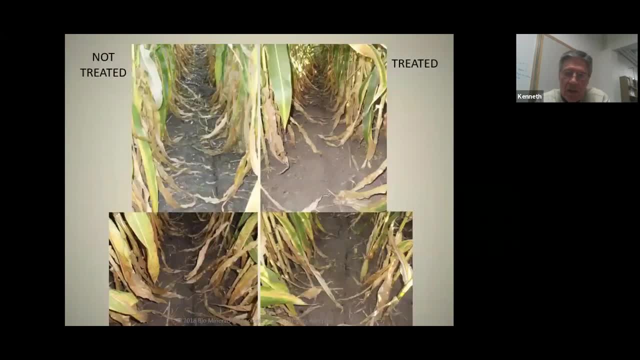 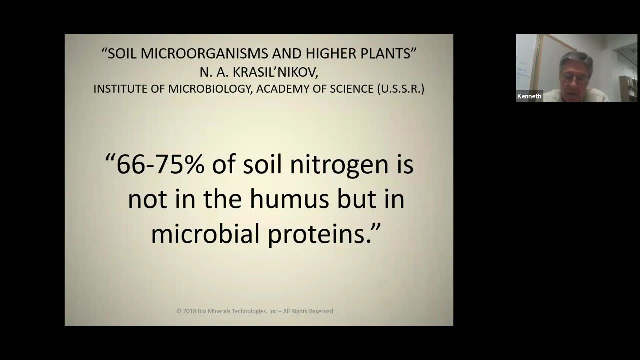 on this particular ear, because the nutrition isn't there. The Russians will tell us that 66 to 75% of the soil nitrogen is not in the humus but in the microbial proteins, And this is again where the microbes hold the mineral content. 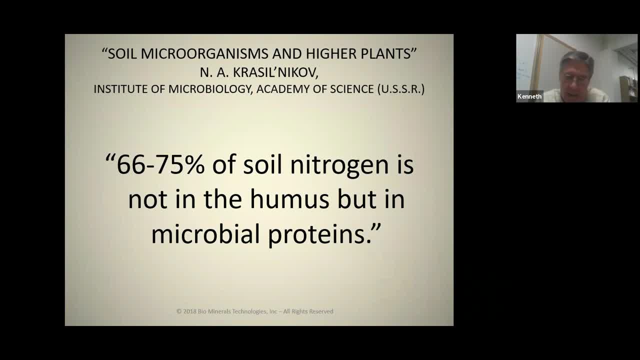 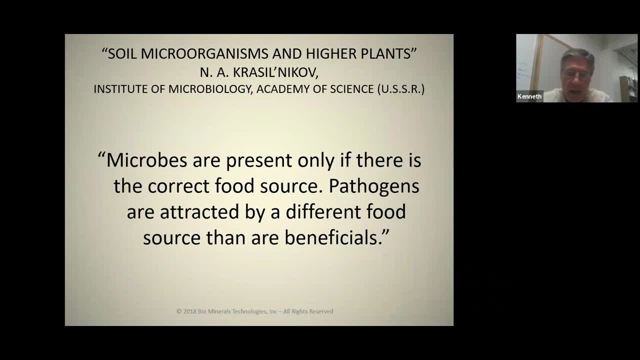 the protozoa come back and eat them and release the minerals for the plants. Microbes are present only if there is a correct food source for them. Pathogens are attracted. They are attracted by a different food source than are beneficial. Again, this is a division in nature, where God does not allow. 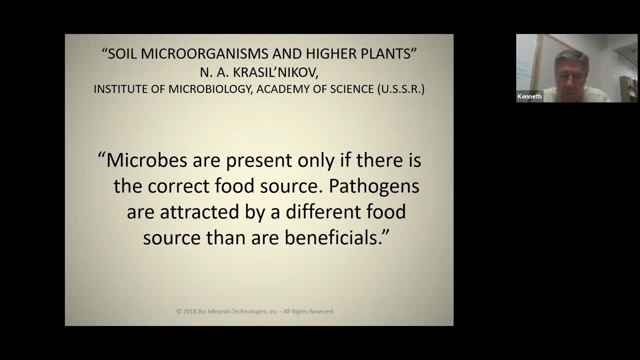 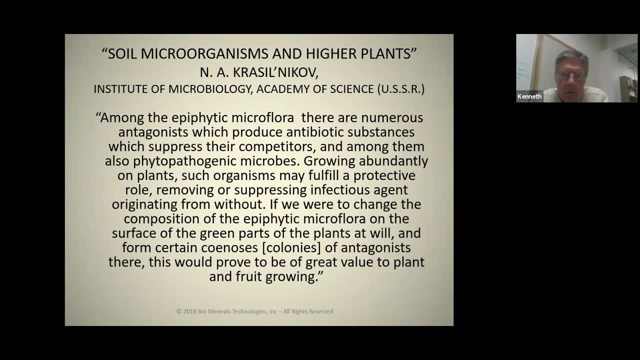 a pathogen and a beneficial to do the same things, And they do not. What this is saying is that we have microflora that are antagonistic. These are the beneficials that produce antibiotic substances to suppress their competitors or pathogens- Soils. 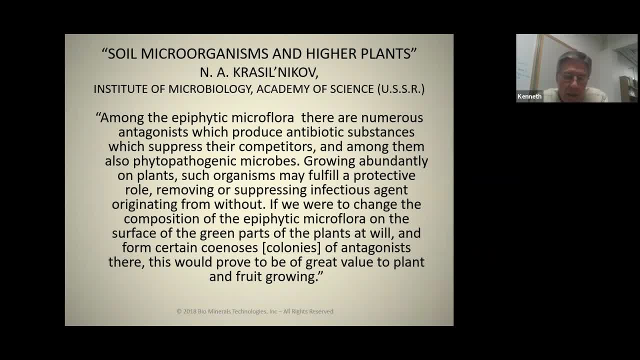 have the ability to govern and control and clean themselves. And so this is to the good guy, bad guy, balancing. And when we put products in that promote the beneficial microorganisms, they expand. When we put products into the soil, that kill the beneficial populations. 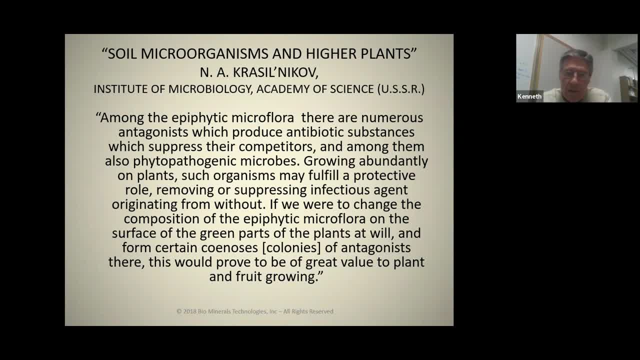 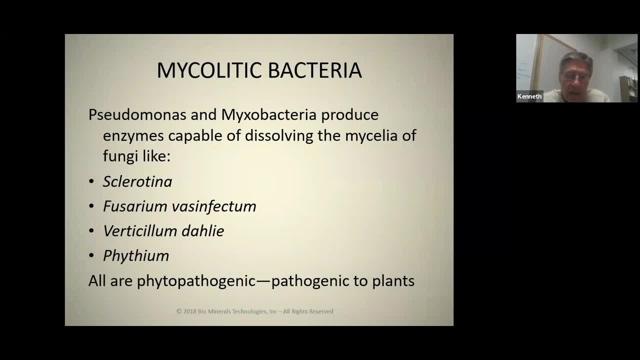 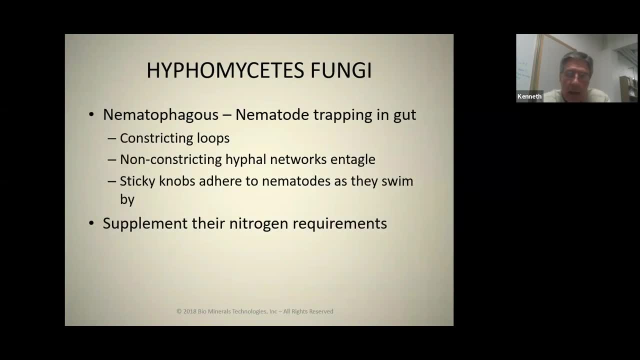 and stimulate the pathogenic populations, we're going to see more disease and less plant production. Then there's a series of mycolytic bacteria that suppress all kinds of fungal pathogens, like Pythium Verticillium Fusarium, And we have pathogenic nematodes that are eaten by fungi. 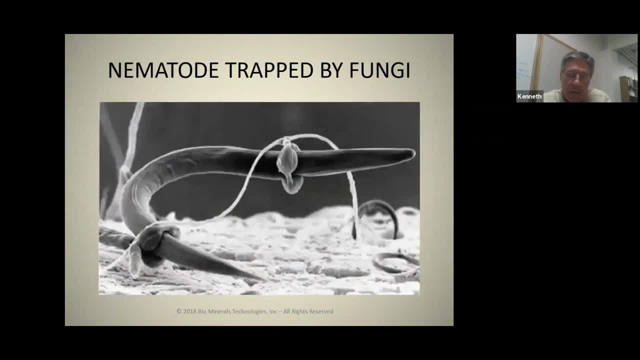 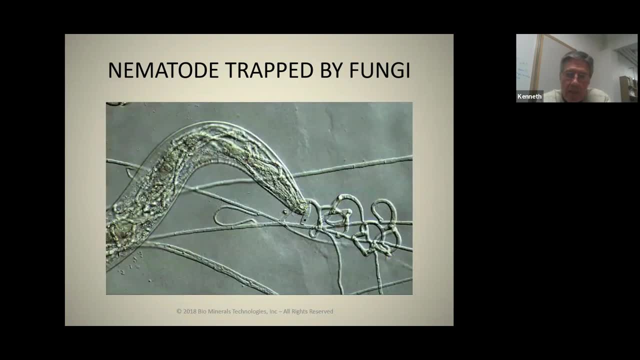 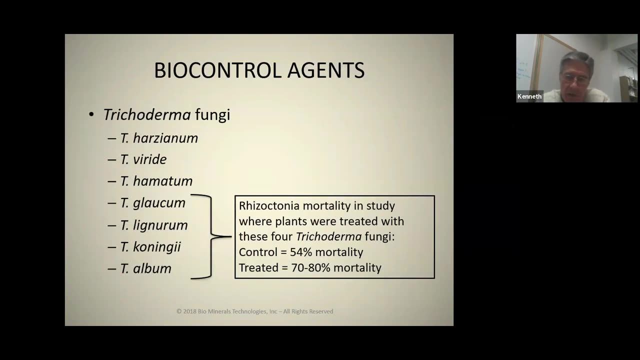 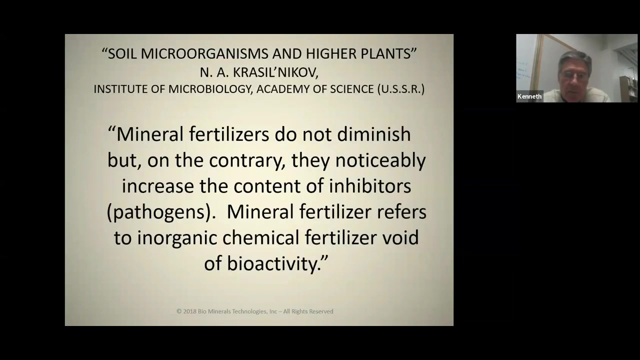 And we have some pictures where you can actually watch the nematode get trapped by the fungi and eaten and removed from the system. Very fascinating process. Trichoderma beneficial fungi are very effective against Rhizoctonia And we have Actinomyces that control a lot of pathogenic microorganisms. 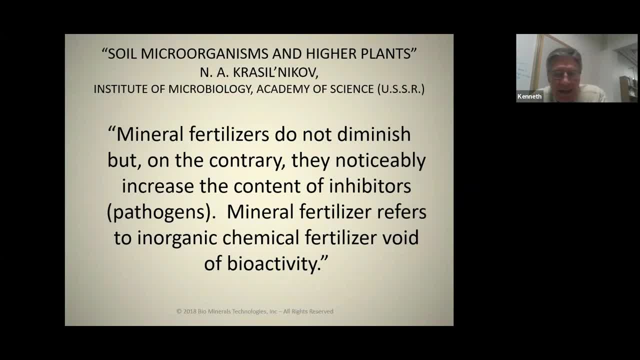 One other thing that we need to be aware of is mineral fertilizers do not diminish but on the contrary, they noticeably increase the contents of inhibitors or pathogens. Mineral fertilizers refer to inorganic chemical fertilizers as a void of activity, So a lot of the refined products that we buy from the fertilizer companies. 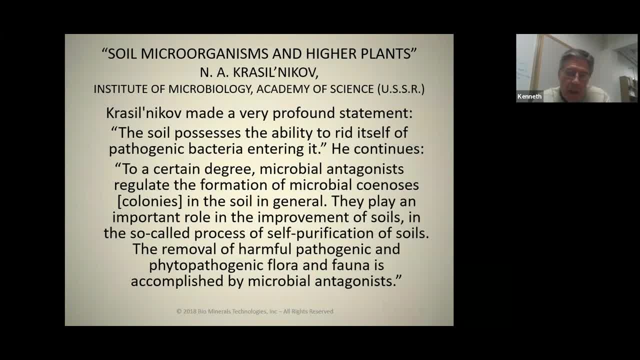 are stimulating the pathogens in our soil out there, And what the research tells us is that our soils have the ability to rid themselves of the pathogenic bacteria coming into it. This is the self-purification process And what I will tell you. we've seen this over and over. 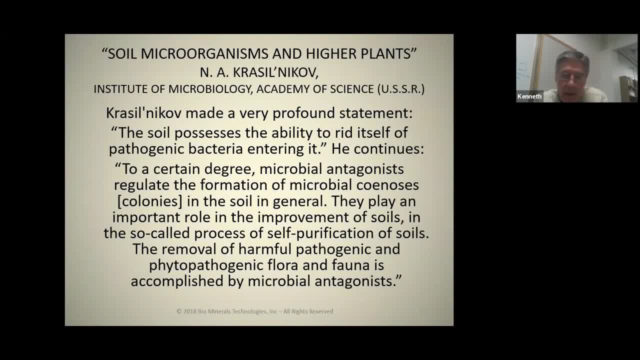 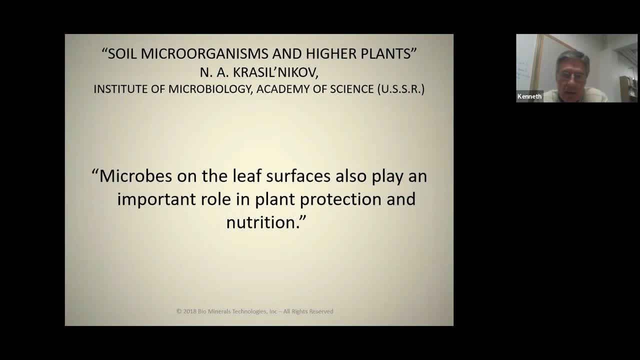 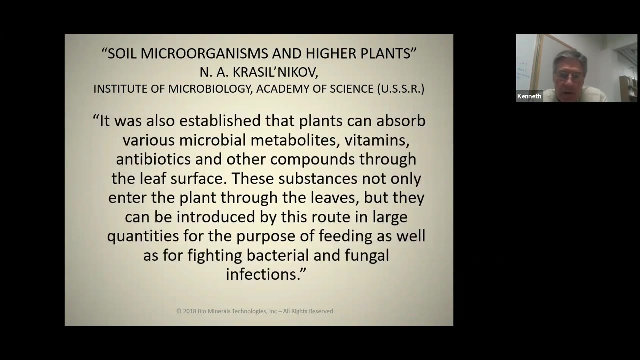 microbial warfare depends upon one factor: He who has the most wins. When we promote the beneficial microorganisms, they keep the pathogens in check. Microorganisms on the leaf surfaces play a role in plant protection and nutrition. It is well established that plants can absorb various microbial metabolites. 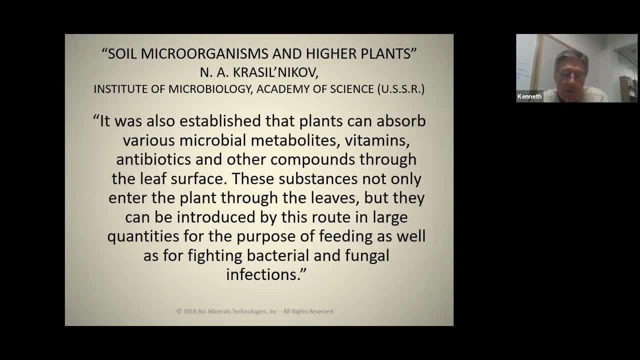 vitamins, antibiotics and other compounds through the leaf surfaces. These substances not only enter the plant through the leaf, but they can be introduced by this route into large quantities for the purpose of feeding as well as for fighting bacterial and fungal infections, And so earlier I mentioned that we have the RIT system. 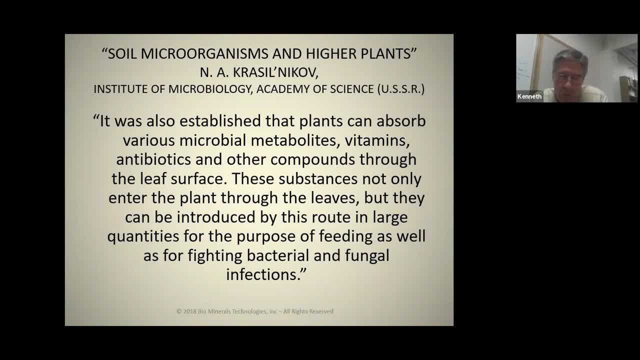 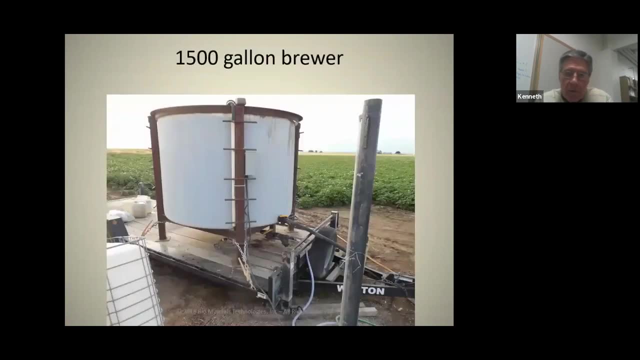 We have the entire foliage that we can put beneficial microorganisms on and grow those colonies. One is a protective barrier against airborne pathogens, but also to produce nutrition from the air- Microbial mineral tea- These are tea brewers that we use. We grow a huge population of bacteria, fungi, protozoa. 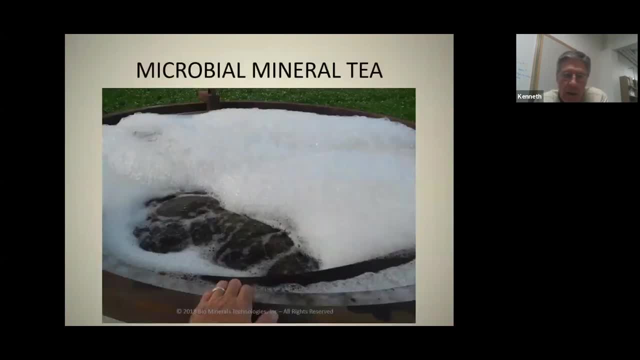 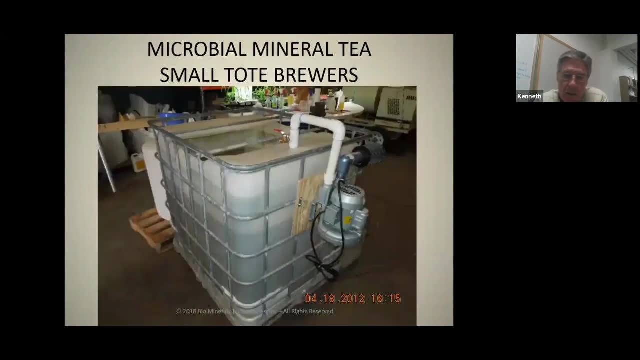 and we put these back out in the soil And this is an amazing process of reestablishing beneficial microorganisms into places that we don't have them or we've altered the populations into pathogenic or unfriendly bacteria. You have large brewers. you have very small brewers. 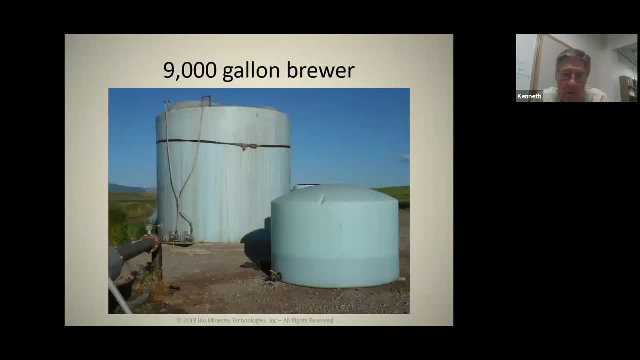 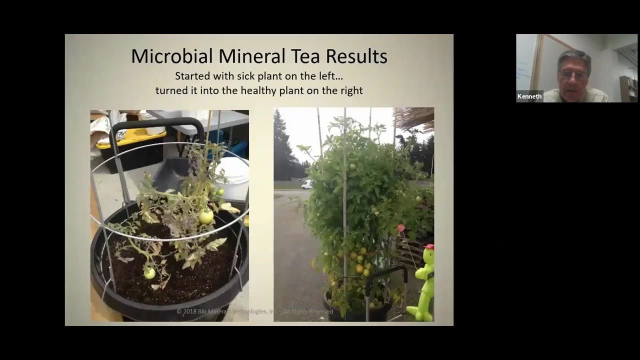 This is a 9,000 gallon brewer that one of our major farms up in Montana uses. They're brewing constantly from about April to October. This goes over about 8,000 acres. This is some wonderful results of microbes and soluble minerals. 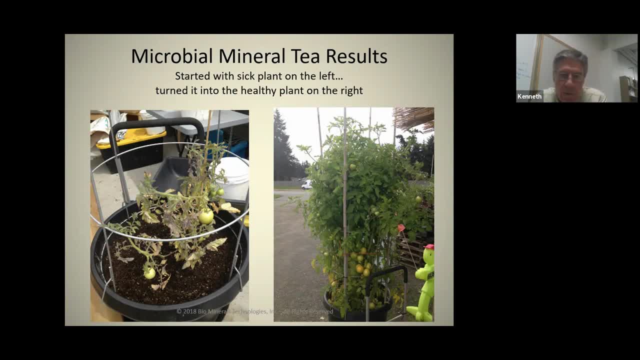 We have some wonderful distributors that work with us up in Washington And they work primarily with gardeners and small farms. This was an abandoned tomato plant. This is microbial mineral tea given to that tomato plant And you can see what a nice recovery it was. 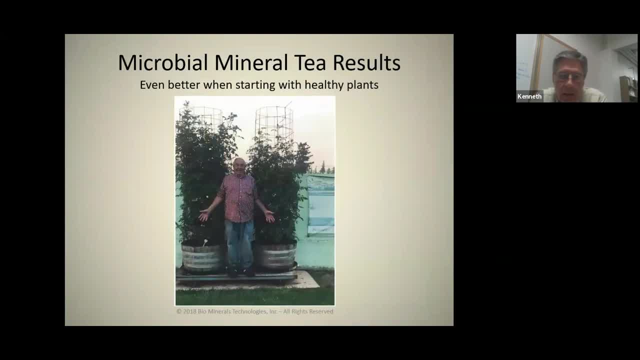 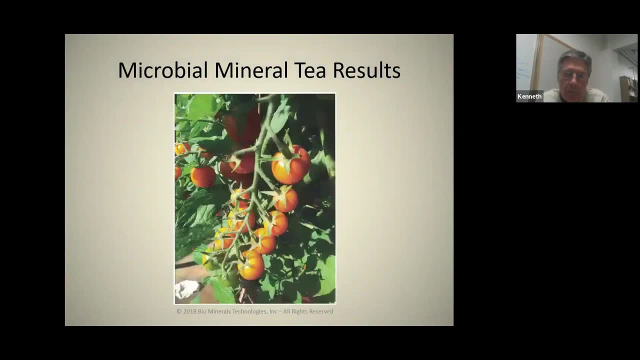 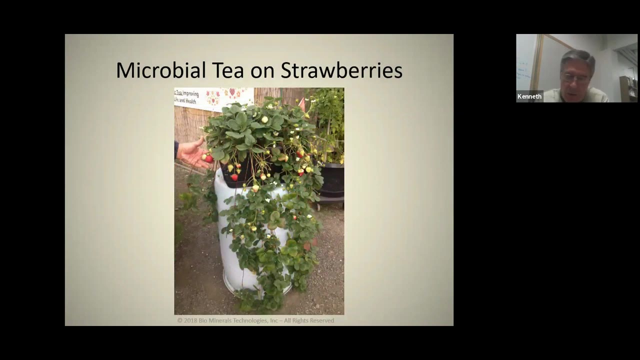 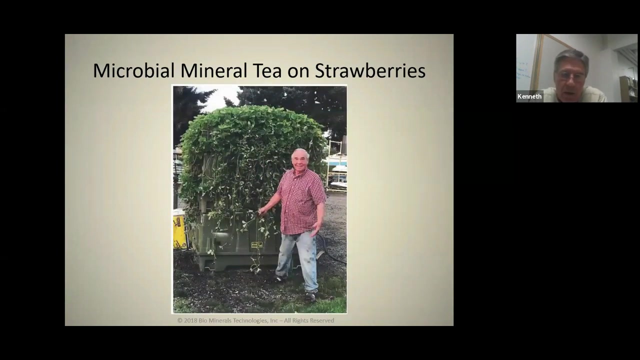 This is Len And these are several of his cherry tomato plants. This is several years ago, one of Len's strawberries. It's on a 55 gallon drum plus about a one foot base. These are Len's strawberries now using biology and mineral tea. 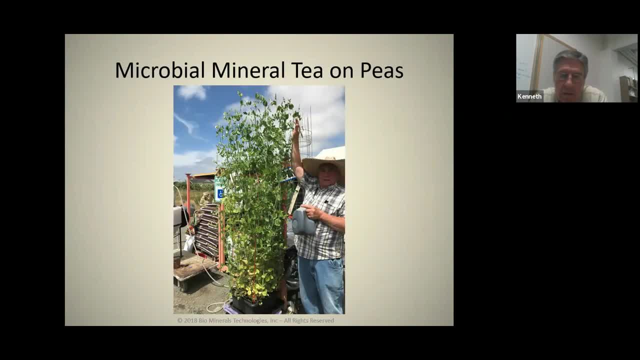 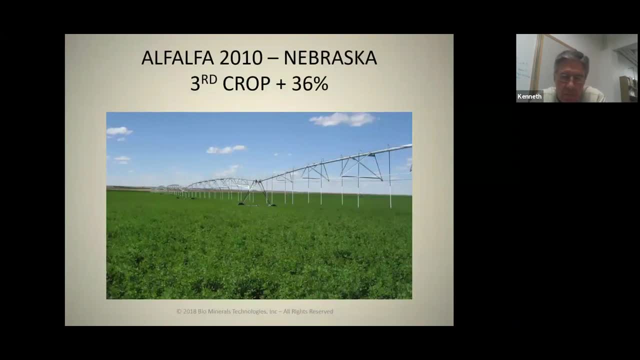 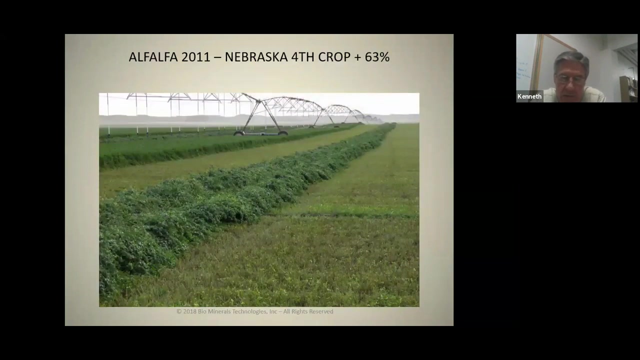 This is Len's pea plant. This is a field that we treated with mineral soluble minerals in Nebraska And we had a 36% increase in the third crop of alfalfa. The fourth cutting that year increased 45%. By the following year we had an increase of 63% in production.